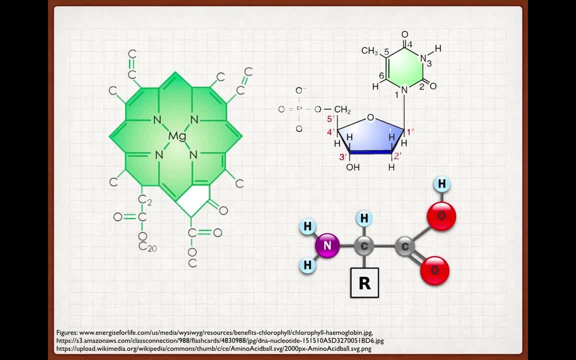 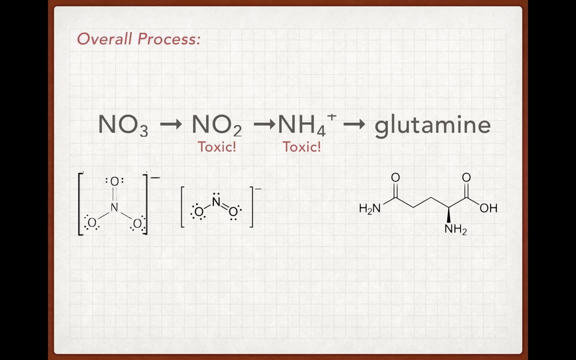 which is done by bacteria. So we know that plants need nitrogen to make things like the chlorophyll molecule or D3., But they also need it for amino acids. So I'd like to follow a nitrate molecule through the plant as it is converted into amino acid: nitrogen. Plants take up nitrate and ammonium. 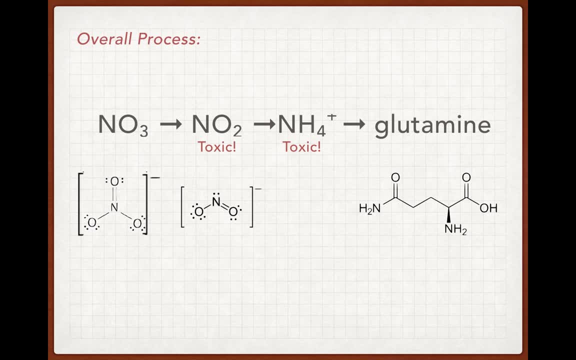 nitrogen through specialized membrane channels, and the process of the conversion of nitrate involves two intermediates, and both those intermediates are very reactive. So the conversion process goes very quickly and the transcription of the DNA that codes for the enzymes that facilitate those reactions is a function of the concentration of nitrogen in plant. 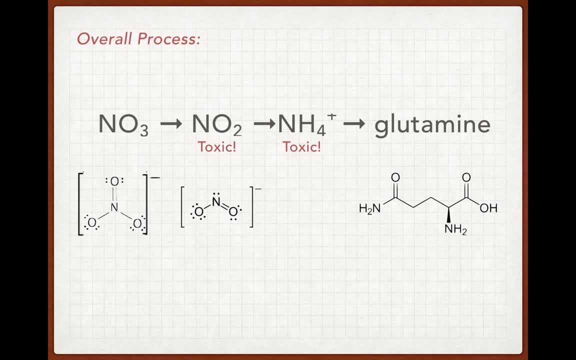 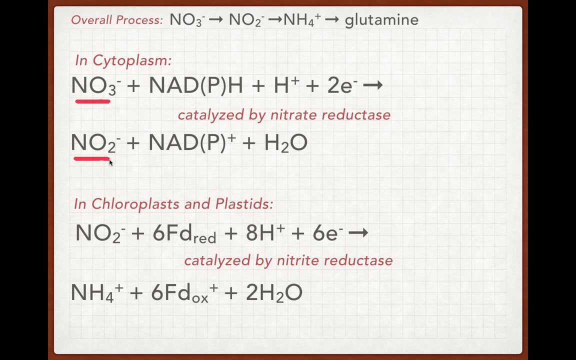 cells to ensure that those reactions happen quickly. So in the first step, in which nitrate is converted to, nitrite occurs in the cytoplasm, with reducing power from NAD8 to NAD46.. Oops, sorry, or NADPH, and it is catalyzed by the enzyme nitrate reductase. The second step because 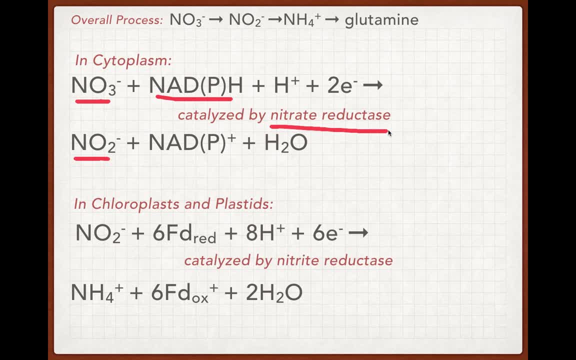 of the reactivity of the intermediates occurs in the plastids, and that's where nitrite is converted to ammonium by the enzyme nitrate reductase, And this occurs with reducing power from ferredoxin or NADH, depending on the part of the plant in which it's occurring. 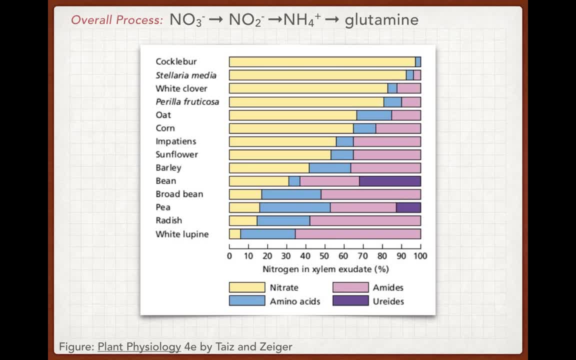 So where in the plant do these things happen? It turns out it depends to some degree on the form of nitrogen the plant is using and also on the species of plant. So here we have the percentage of different forms of nitrogen found in the xylem, and you'll see that it 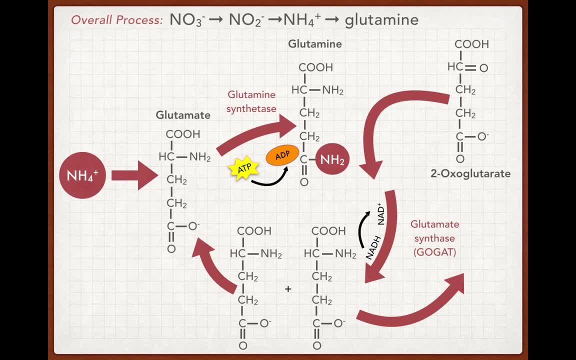 varies quite a bit with plant species. Okay, so here's the final step, where we go from ammonium to glutamine, and this can actually happen through the process of the process. So we go through a number of metabolic pathways. This is one called the GOGAT cycle, and you'll